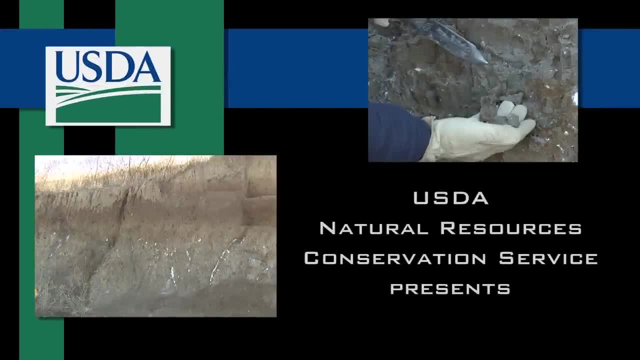 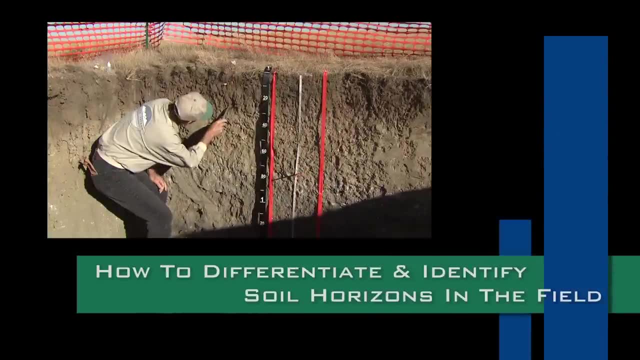 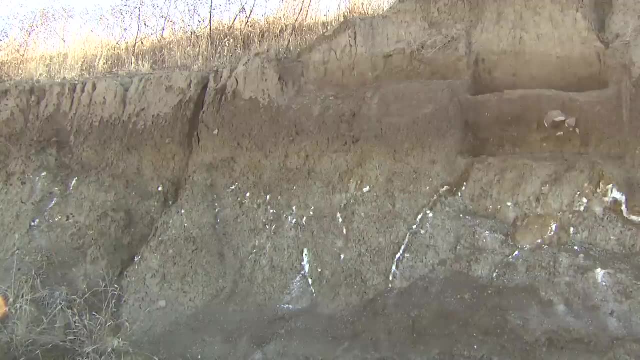 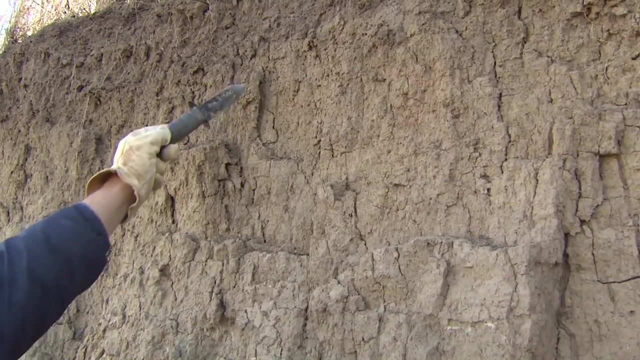 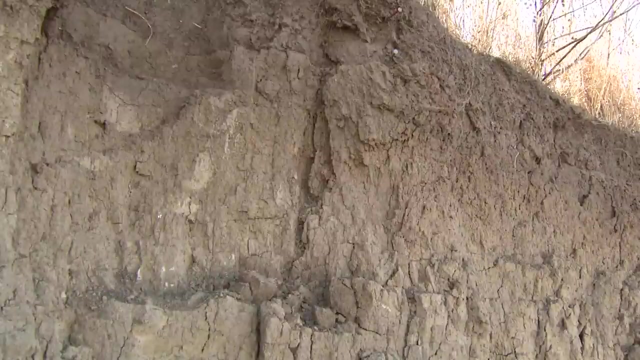 This job aid is designed to help you differentiate and identify soil horizons in the field. After viewing this video, you should be able to follow the National Cooperative Soil Survey methods to independently identify soil horizons, their depth and boundaries between them, and understand the observation method used to describe soil horizons. 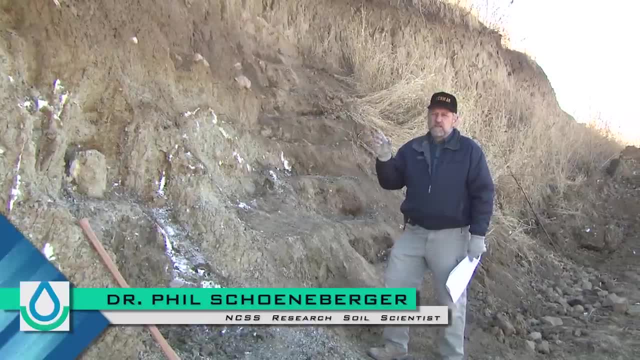 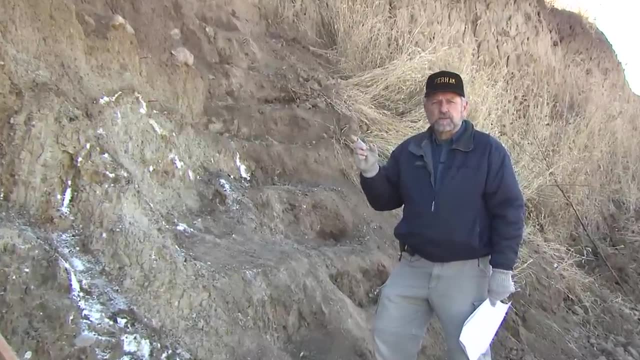 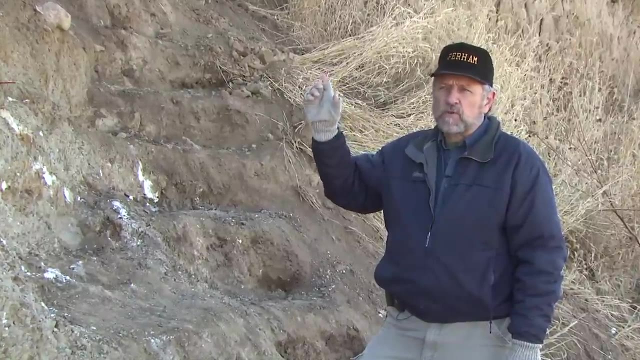 When describing horizonation, the most important items are just basics which you already know. Describe and record what you see. We're interested in trying to capture the main layers or horizons or stratigraphy that we find in any exposure. The larger the exposure that you have to make. 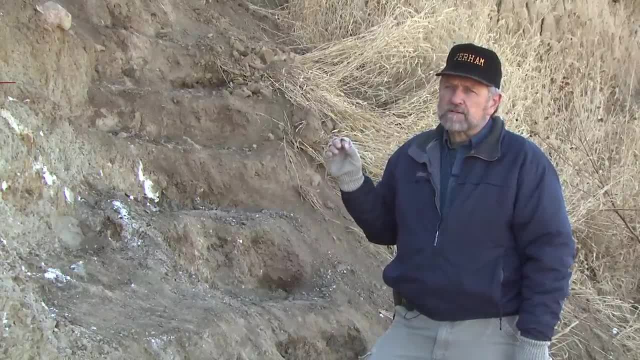 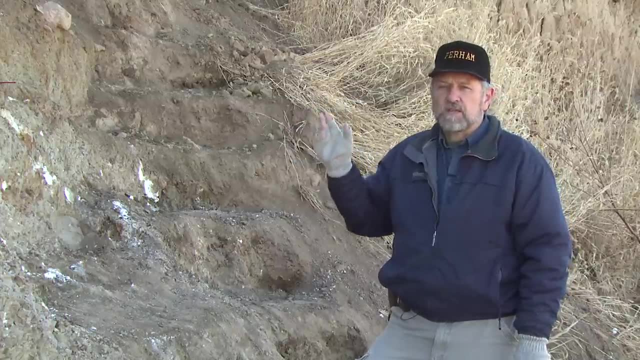 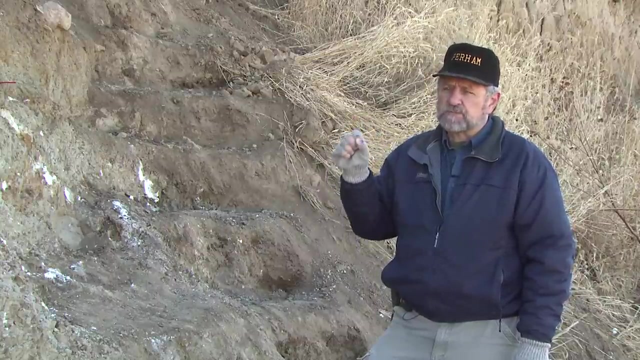 observations, the better job you're going to have in understanding the context of what it is you see. So when you find large exposures like this, take full advantage of them- road cuts, basements, pipeline banks, whatever you can find- because that helps explain what. 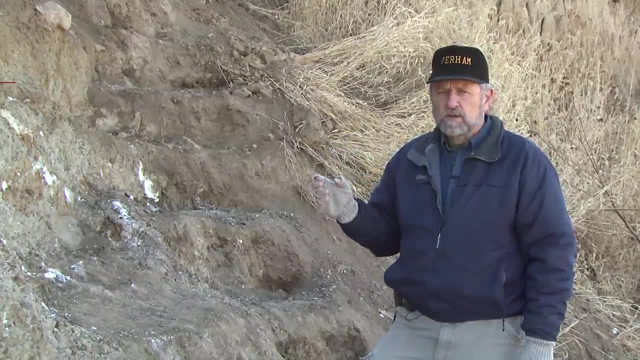 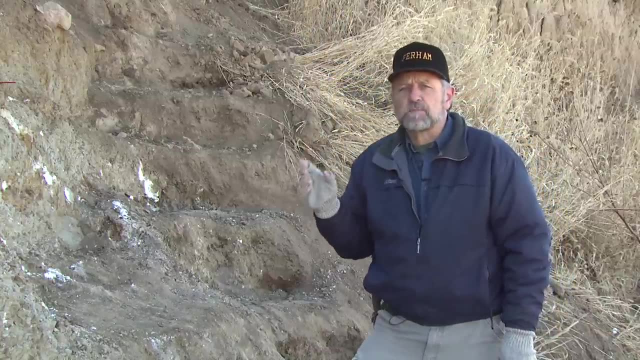 you see, in much smaller sampling, that you typically get out of a pit or out of an auger hole When you first look at a site and begin to evaluate it. most people are interested in picking out the obvious things. You want to pick out color changes, because they're usually 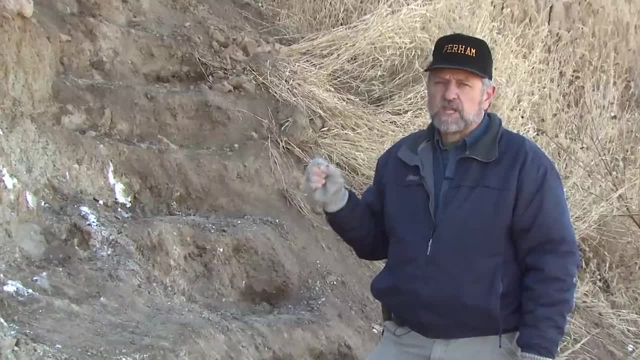 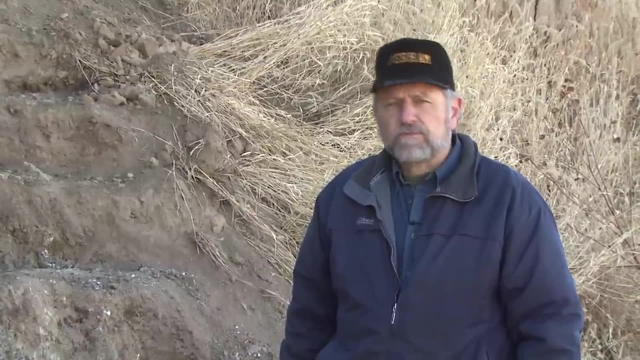 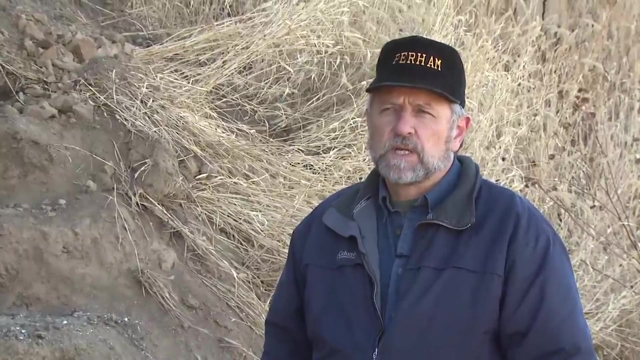 the easiest to see and focus on. The last thing you want to do when you're done is actually label the horizonation. Many people will do that first, and that's unfortunate, because you'll bias yourself and not see things or pay attention to things that you should. So 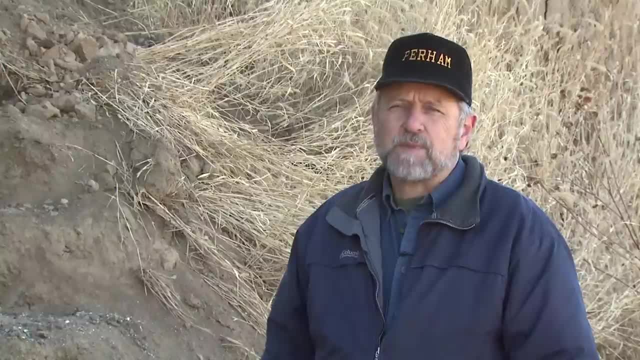 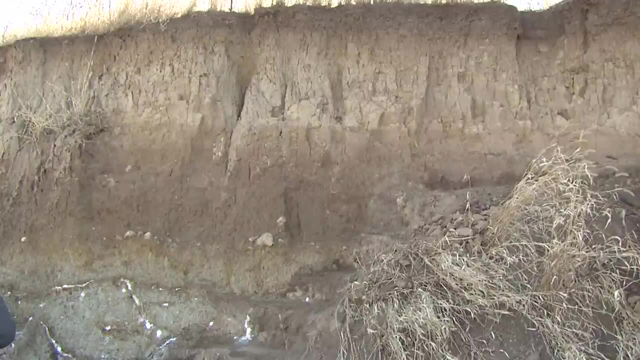 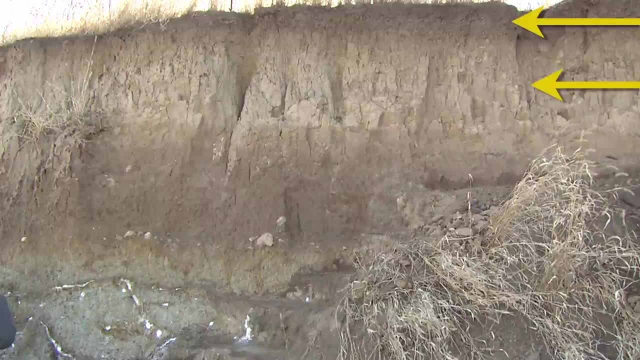 start with a clean slate. Save the horizonation naming to the end and just focus on the layers and the features that you find. So if you look at this site, we've got a number of different zones and you can see color differences. There's something dark up top. It gets brighter and grayer as 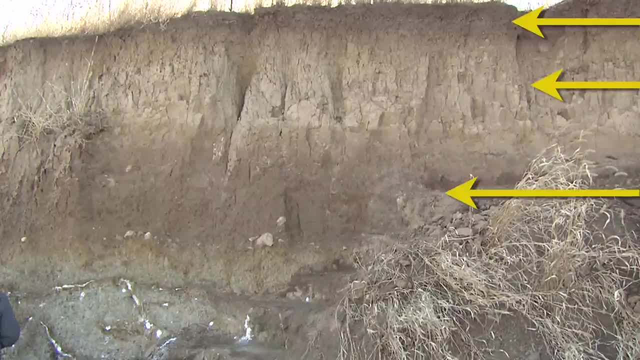 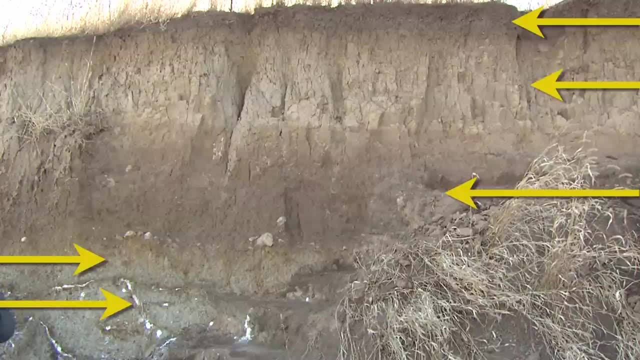 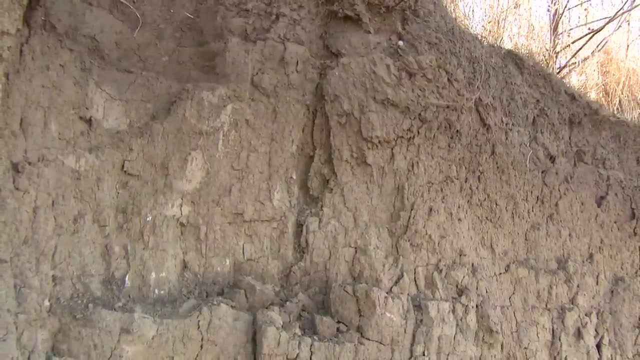 you come down the face, Then you have a chocolate brown layer in the middle. You have something gray and some stones down here and these white seams. Those are easily separable into major layers. You split the major layers first because you can come in later, and then subdivide into. 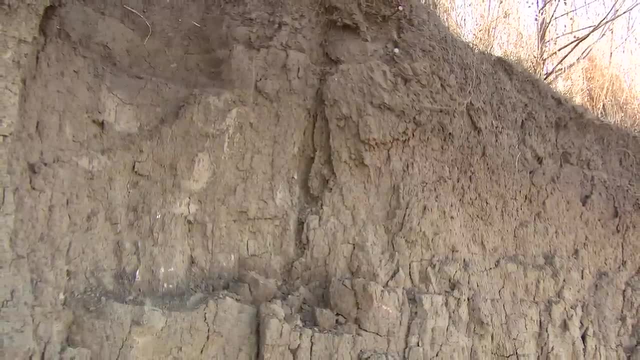 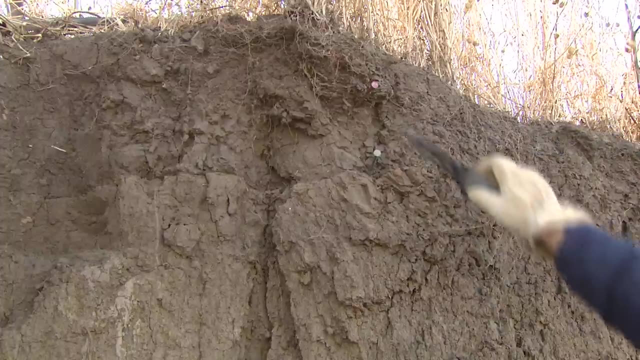 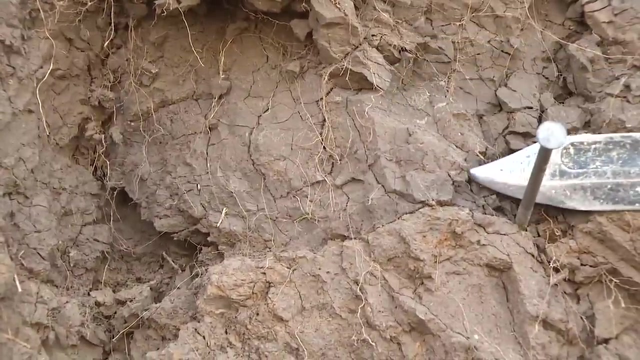 minor layers based on other attributes, whether it's coarse fragments or changes in rooting habit, or whether soil changes in structure. But the main layers are the ones you want to get first, Get the easiest ones and you can come back in later and subdivide And 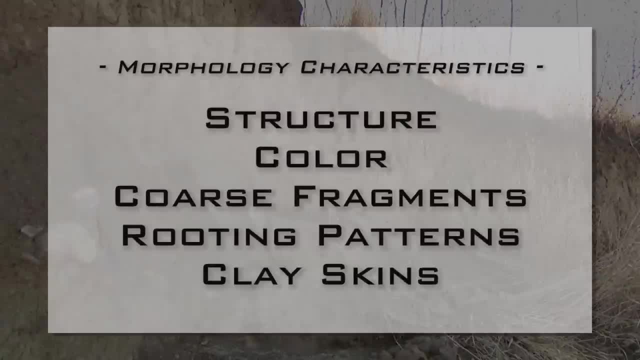 then, as you work through each major morphology- character, structure, color- and then you'll see that you've got a number of different layers that you can subdivide into minor layers And then you can come back in later and subdivide, And then, as you work through each major morphology, 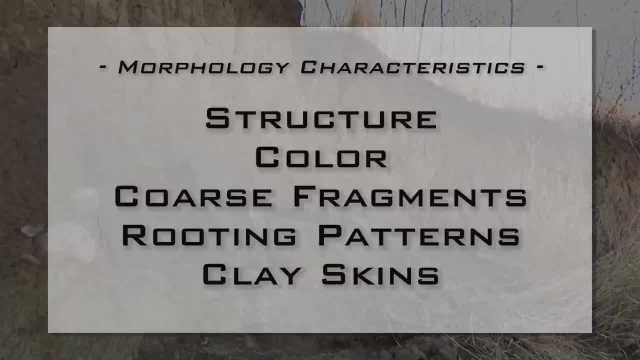 you'll see that you've got a number of different layers that you can subdivide into minor layers. So you'll see that you're flavorings, coarse fragments, rooting patterns, clay skins, presence or absence, all these different descriptors. they will add to the body of information that at the end you can use to give a good solid. 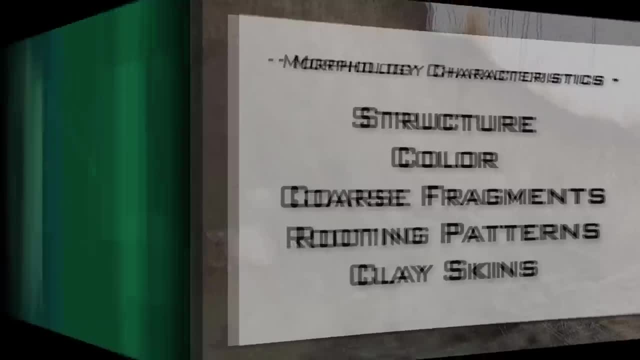 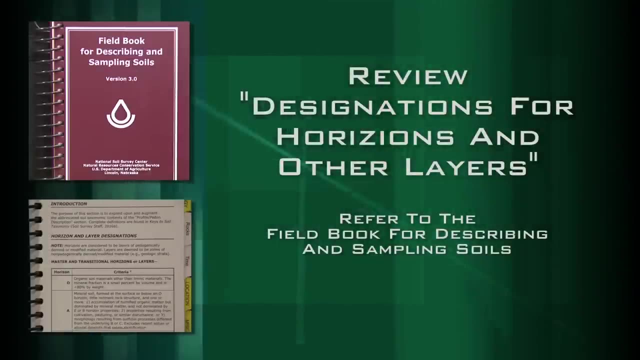 defensible nomenclature for those different layers. Narrator. Now, before you get started in the field, take the time to review the sections of the soil survey manual on designations for horizons and other layers. Refer to the field book for describing and sampling soils, focusing on the charts and. 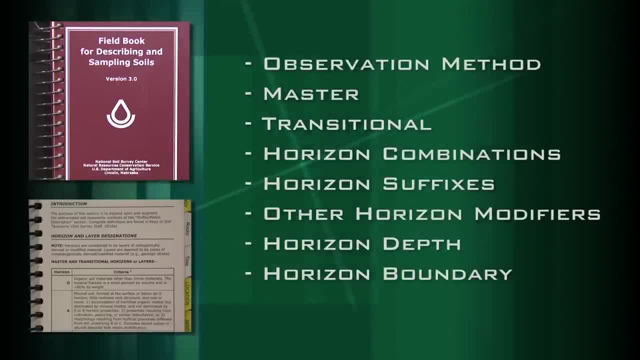 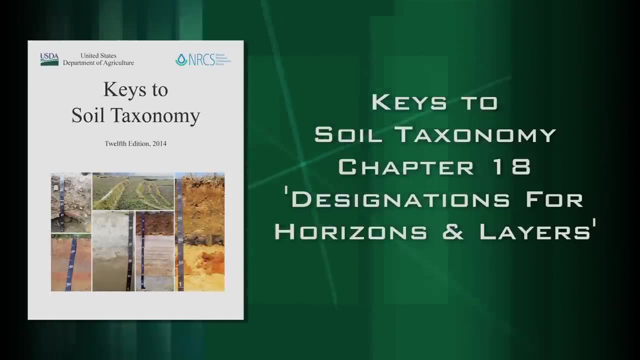 discussions for the observation method: master, transitional and common horizon combinations, horizon suffixes, other horizon modifiers, horizon depth and horizon boundary. The most up-to-date nomenclature for describing soil horizons will be found in the current edition of the Keys to Soil Taxonomy, Chapter 18, Designations for Horizons and Layers. 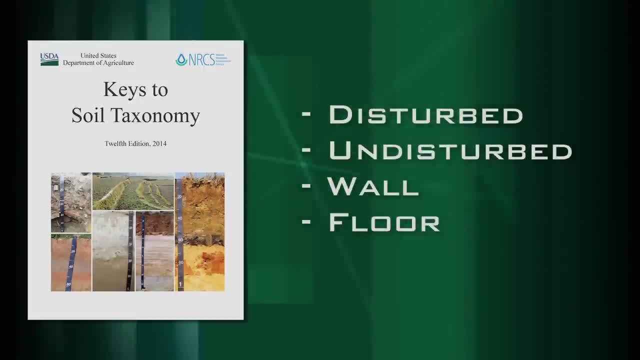 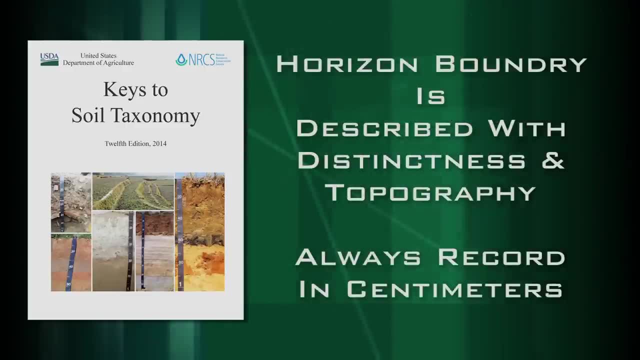 As you review these references, notice the observation methods recorded for disturbed, undisturbed wall and or floor. Also notice that the horizon boundaries is described with a distinctness and topography. Depths and thicknesses should be recorded in centimeters. 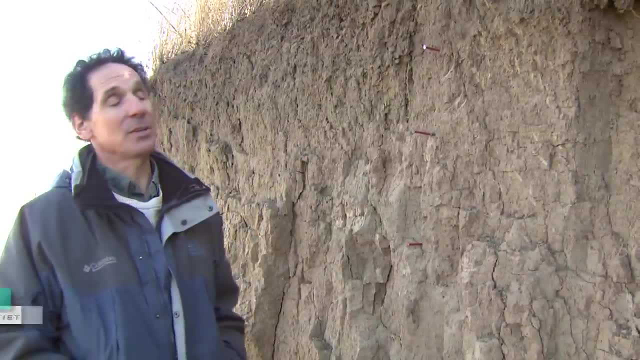 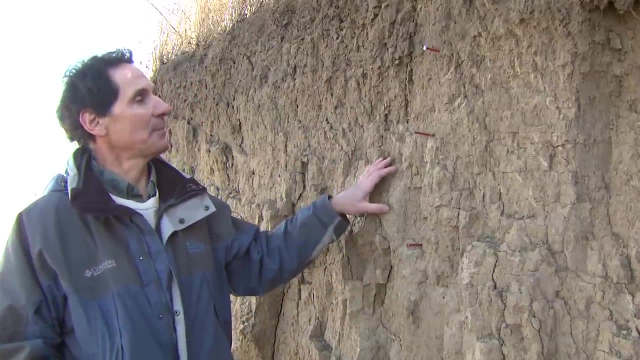 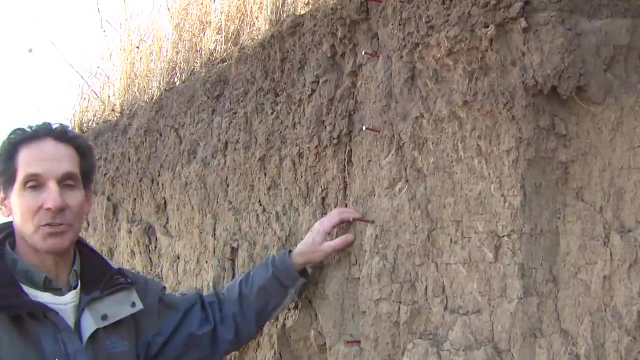 The most important thing to do when describing a soil profile is to describe what you see. In a large exposure here, like we have, it's very obvious to see gross morphology such as soil structure. It's very easy to see soil color and root distribution patterns. 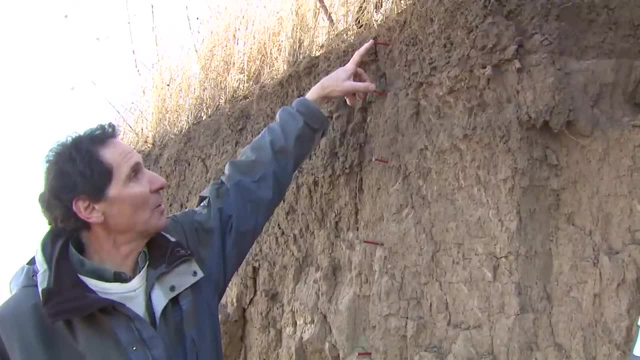 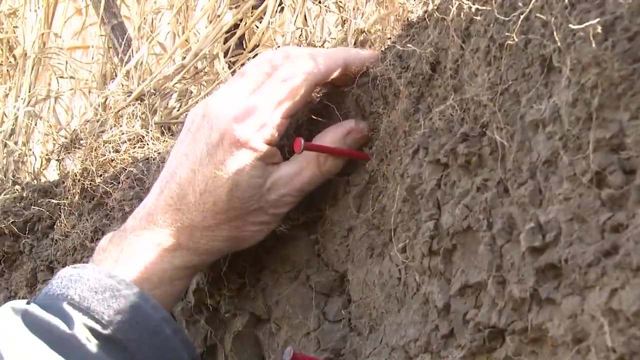 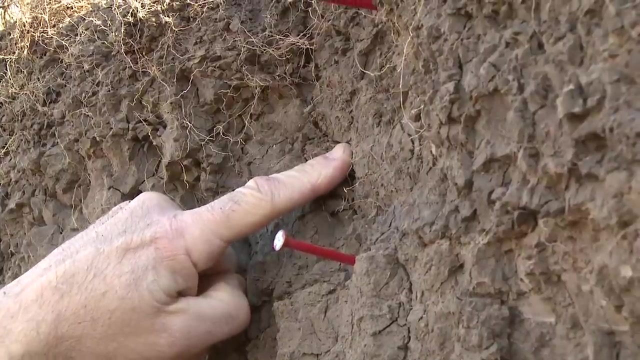 So the breaks that were placed by these red pins mark horizon boundaries that were separated on this morphology. Here we have platey structure, here we have angular blocky structure and a difference in root distribution. This horizon boundary was placed here because we have an abrupt, smooth boundary between 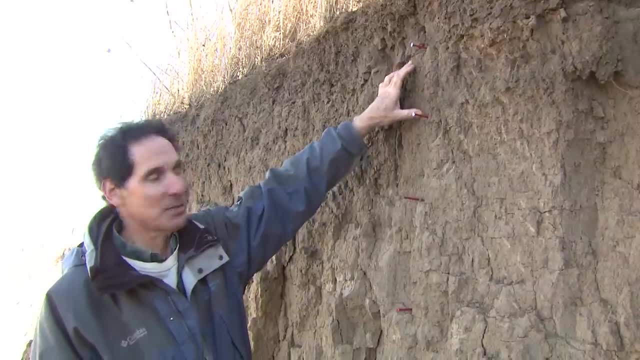 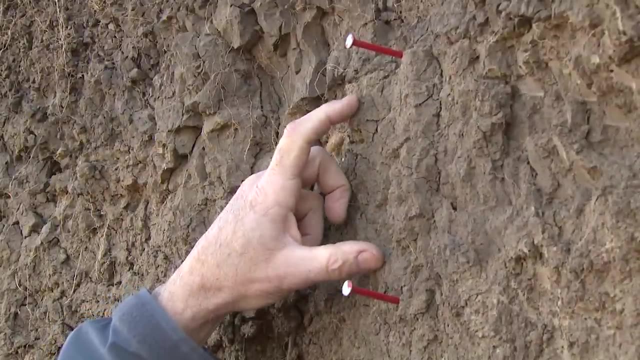 this horizon and this horizon. This horizon has the beginnings of what we call prismatic structure, where we have elongated peds, as does this horizon, which is much browner. You can see this horizon has a different color than this horizon. 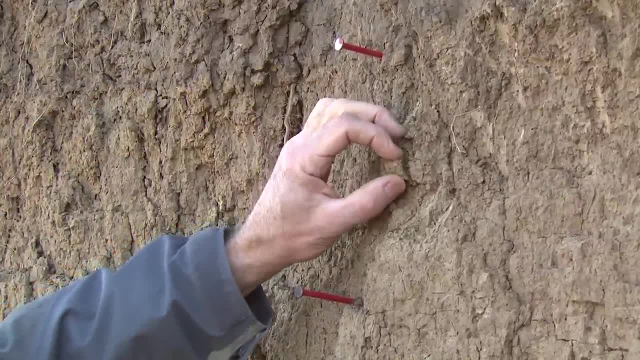 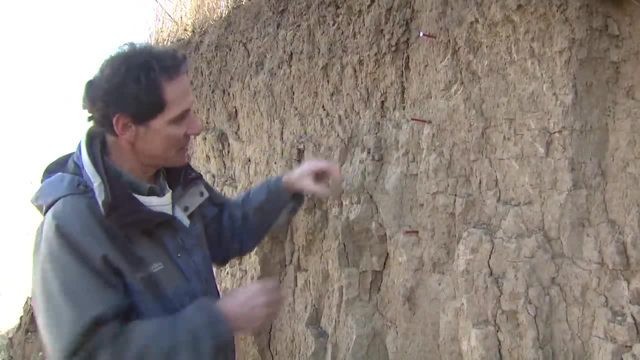 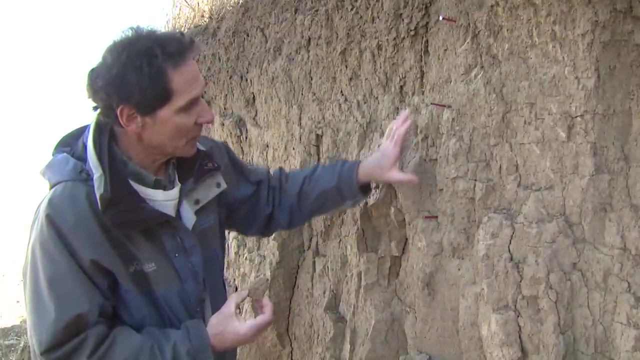 This was broken out based on color and on structure. As we proceed down through the profile, the structure becomes much larger. We get coarser size and longer prisms. This boundary here was placed because of the size difference in the prisms between this. 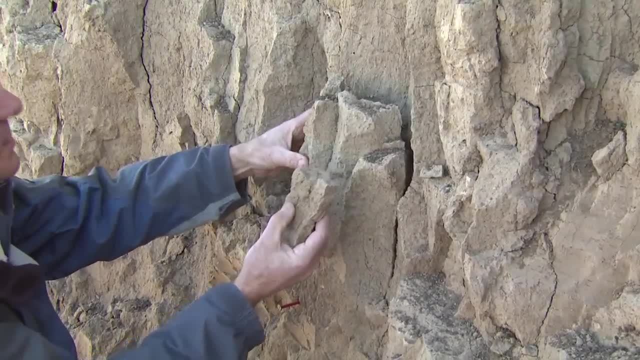 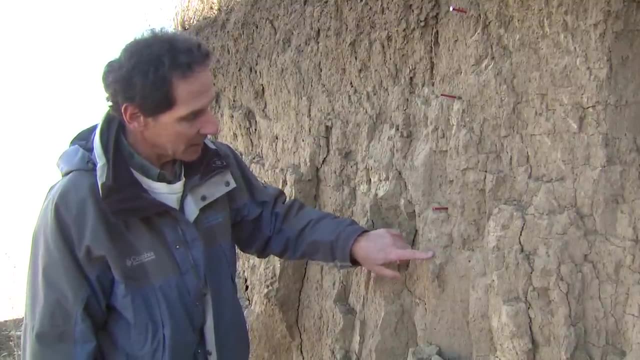 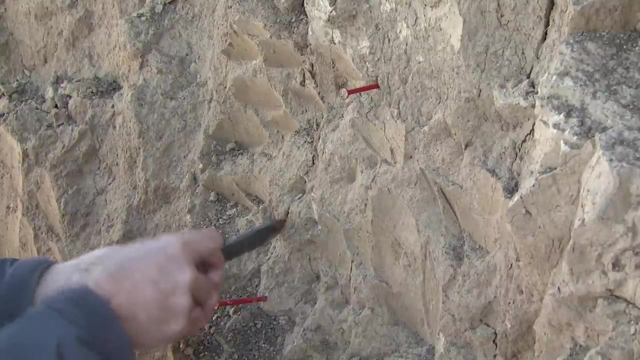 horizon and this one. It was also placed because we see a difference in redoxomorphic concentrations or there, these reddish, orange masses of iron and manganese which are distributed in the profile And then farther down. we have a lithologic discontinuity at this break between another. 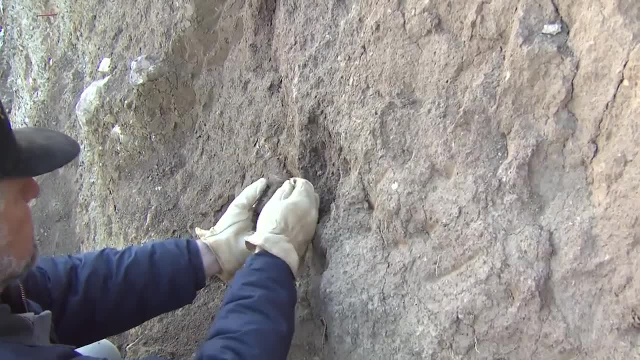 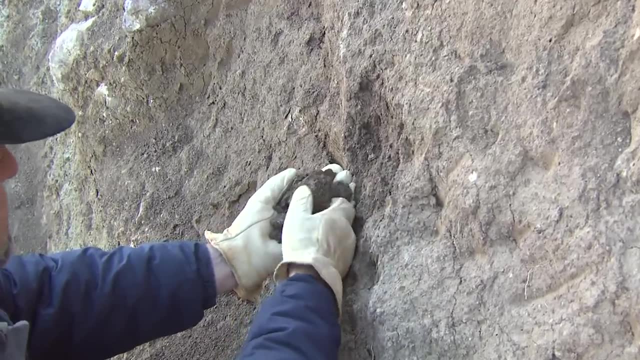 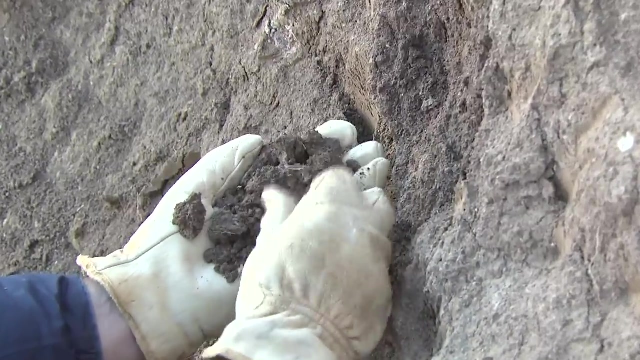 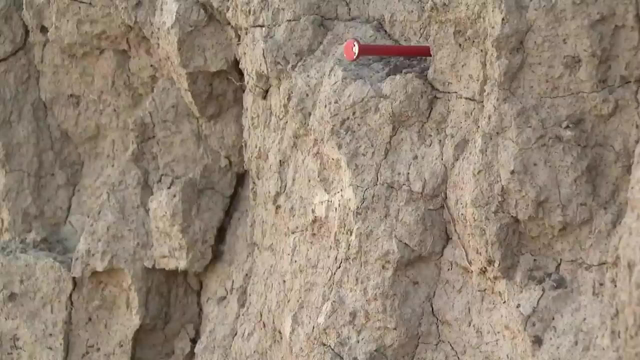 parent material and the structure is obviously different. it's not as well expressed down in this horizon as it is up in here. So as we make these, as we separate the horizons with these initial breaks, then we have to look at the peds more closely to look for soil features such as clay films or secondary 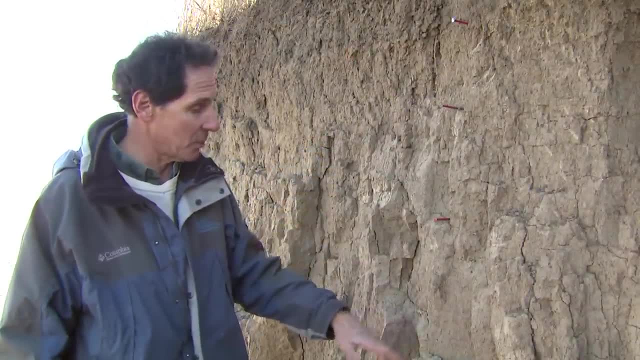 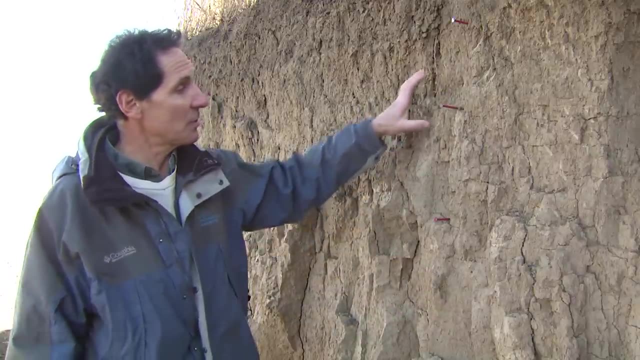 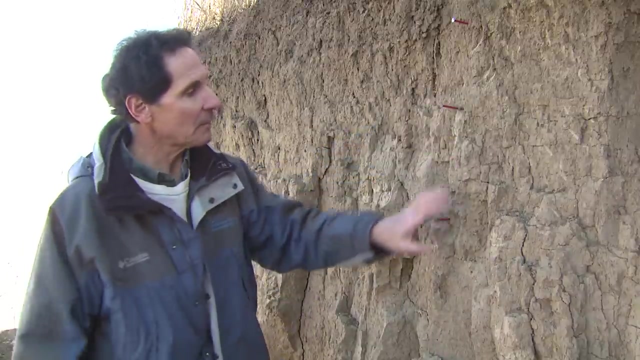 calcium carbonate and the redoxomorphic features which are evident in place in this horizon, but in some horizons you need to remove peds to observe them. So the horizon boundaries can be separated. They can be adjusted as you examine the soil more in depth. 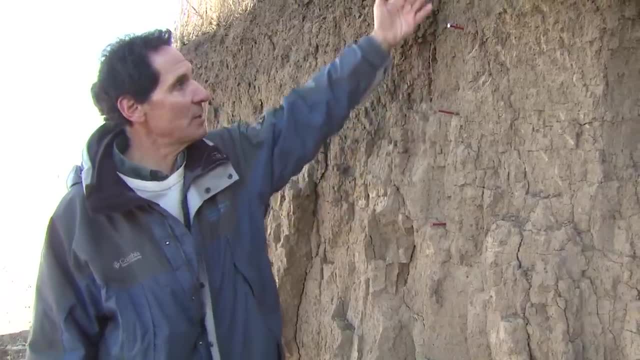 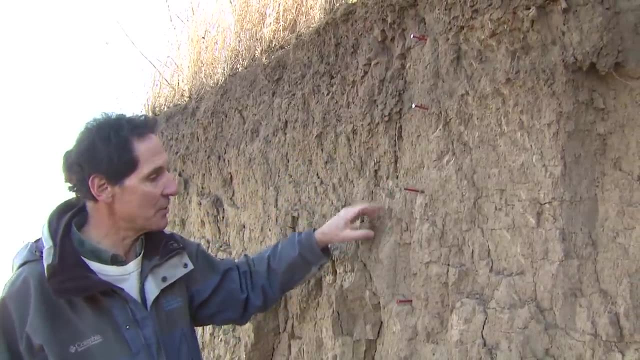 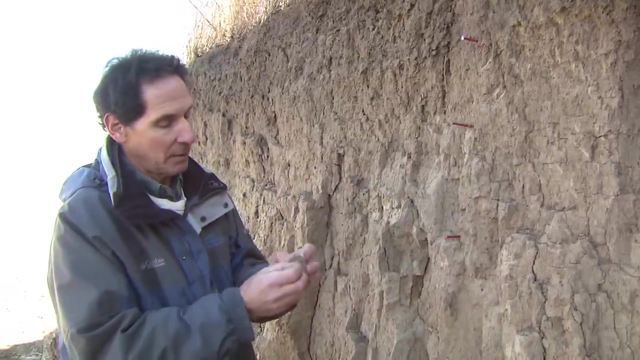 In the case of these horizons here we know that there is alluvial clay that has been redistributed from the surface and alluvied or moved in solution down into these horizons, and it's obvious when you remove some of the prisms and look at their faces. there are coats. 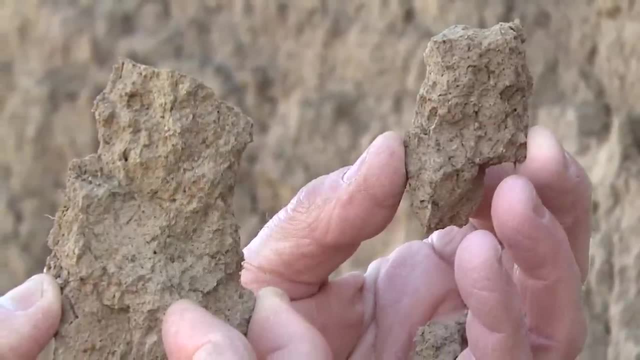 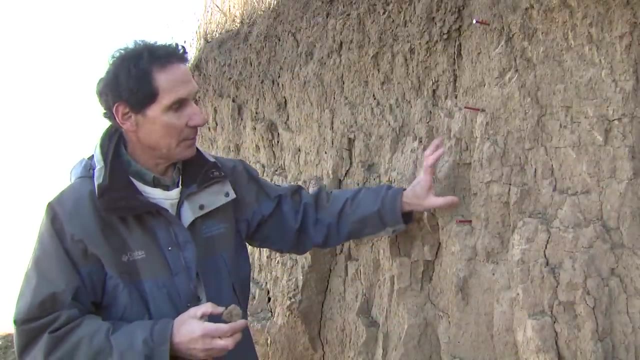 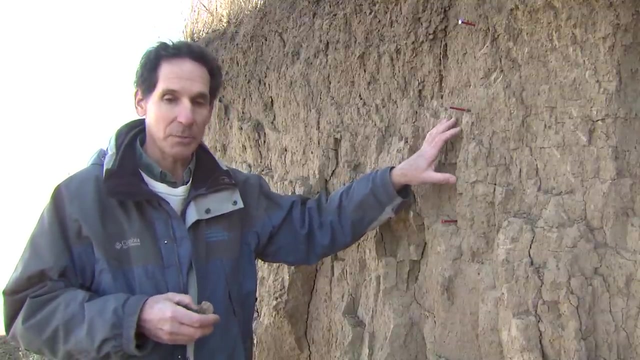 of clay on the faces of the peds And the clay film, the clay filings which are described for each horizon that they occur in, and the presence of those clay films is one of the pieces of evidence that you use to identify this as a master B horizon, and their little suffix T indicates that there. 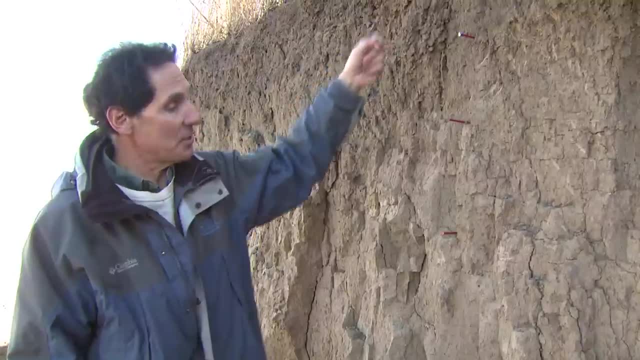 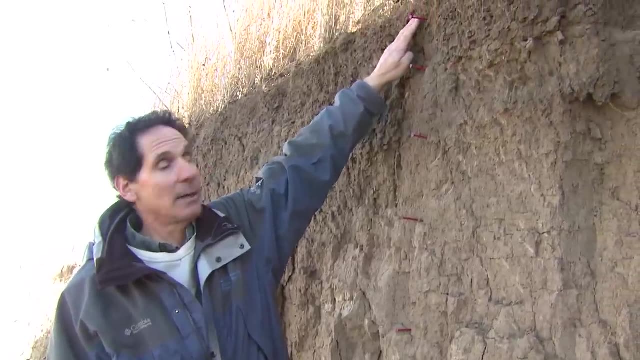 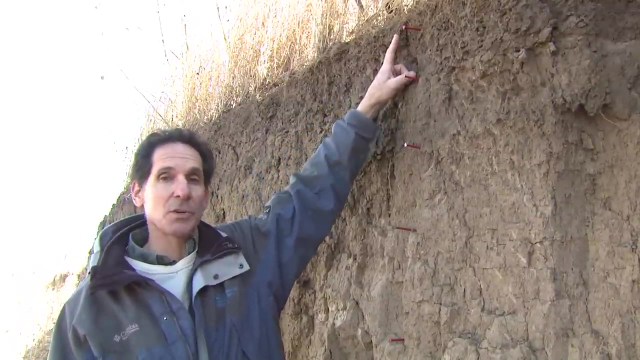 is alluvial clay present. The horizon designations that we gave to the part of the profile that we see here is: the is A master A and two master A horizons, both of which have been disturbed by plowing, So we call that an AP1, and this horizon is an AP2.. 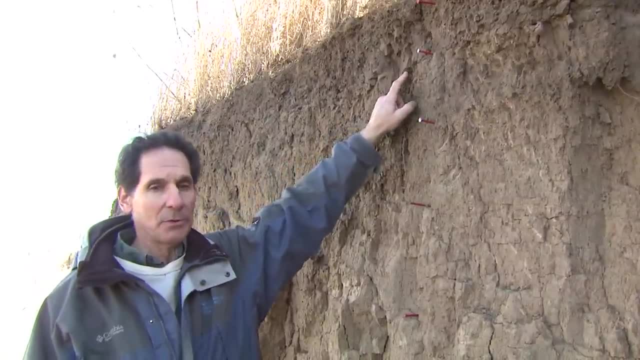 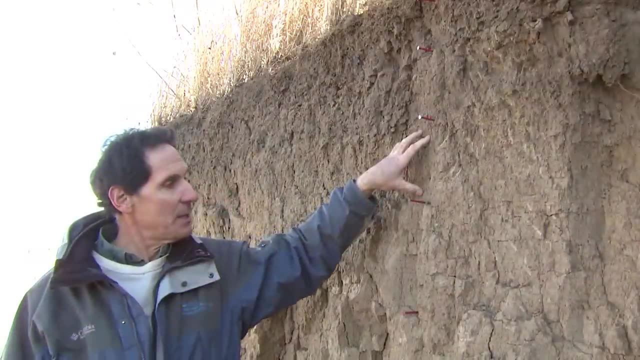 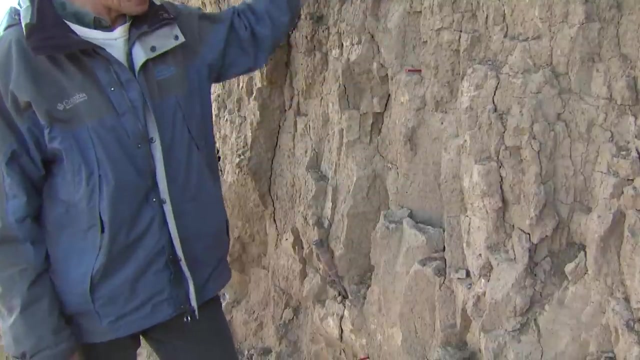 The plowing is the reason that there is an abrupt, smooth boundary here between this AP2 and this BT1 horizon. This horizon here we designated BT2.. This a BT3, and this a BT4. There was no calcium carbonate present in any of these horizons. 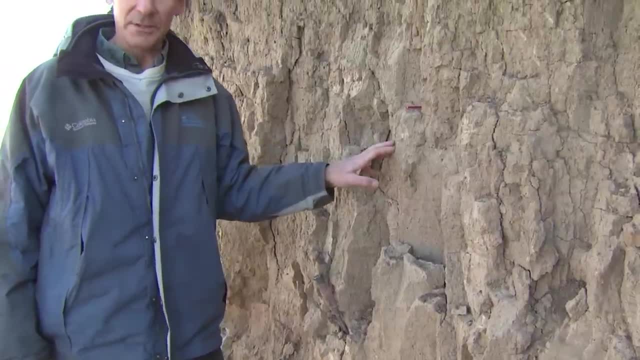 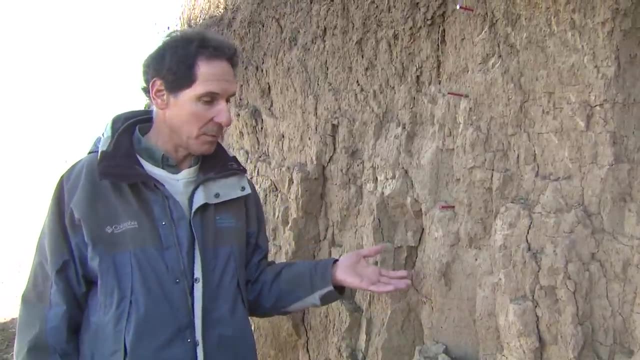 They were non-effervescent throughout, as we used hydrochloric acid to test for the presence of carbonates and there was none, And there's no calcium carbonate that's visible as secondary features. So there's no suffix K on any of these horizons. 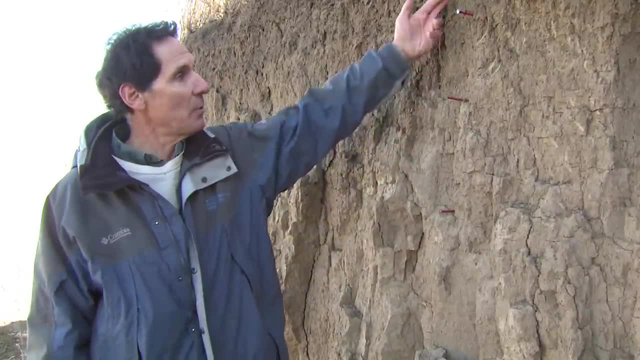 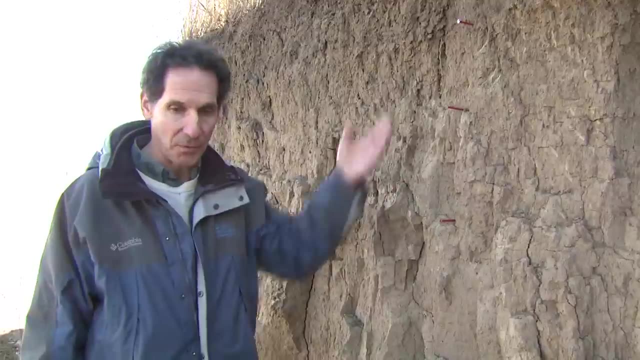 but they do have clay films present. So every one of these B horizons is a, B Is a BT, a BT1 through BT4. So there's a vertical subdivision with depth And then at this pin here we have a lithologic discontinuity. 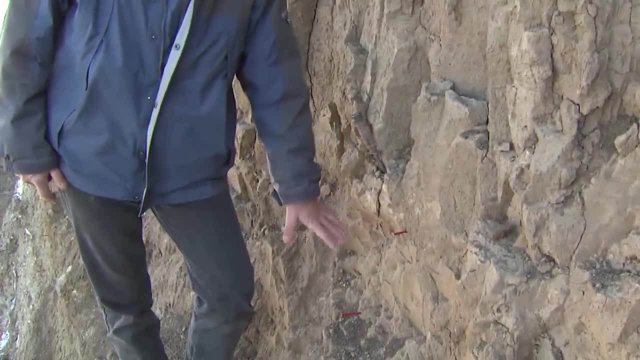 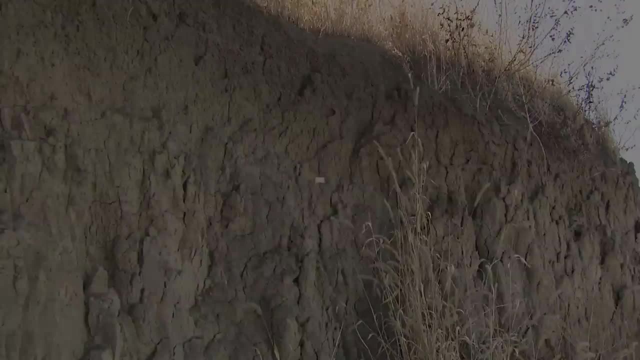 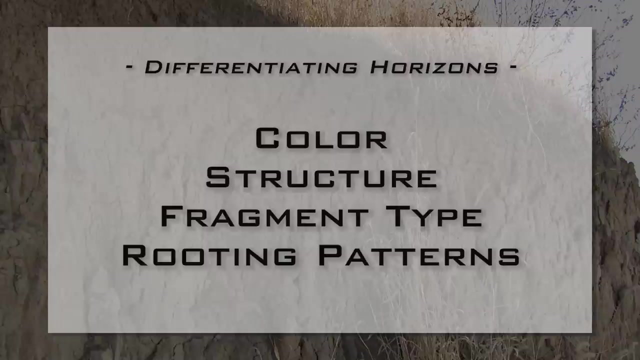 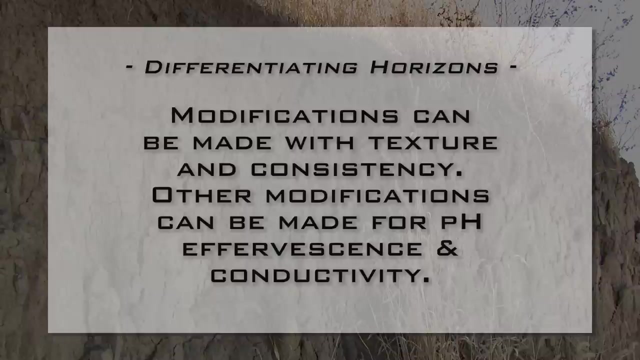 to the next body of soil material which is present from here down for about another meter. To differentiate horizons, start with what is most obviously seen, such as strong differences in color, structure, amount or type. Then set the average intensity on the B horizon. 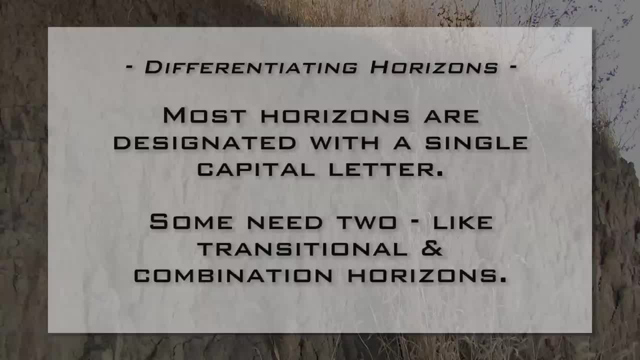 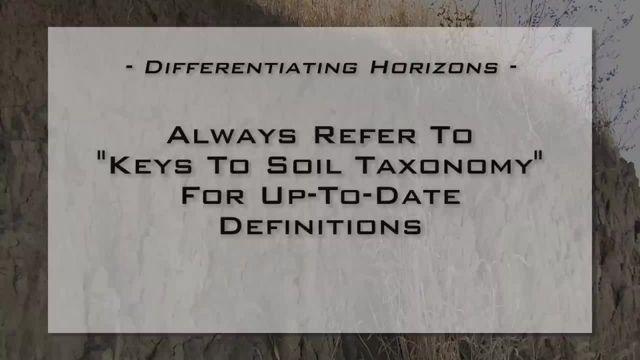 The Keys to Soil Taxonomy contains the most up-to-date definitions of master horizons and their lowercase letter suffixes, numbers and symbols, and the conventions for listing these when used in combination with each other. Review this data focusing on horizons typically used in your survey area. 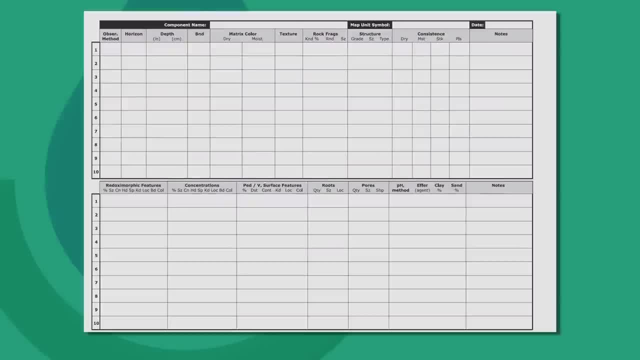 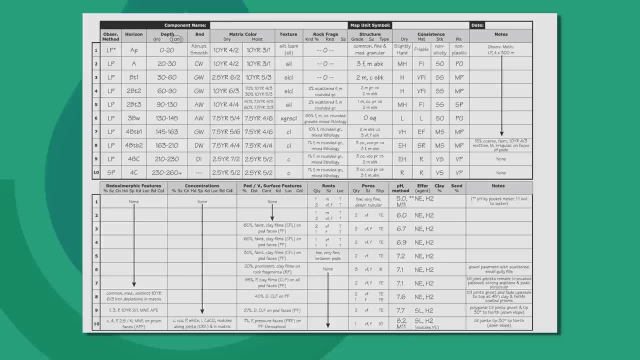 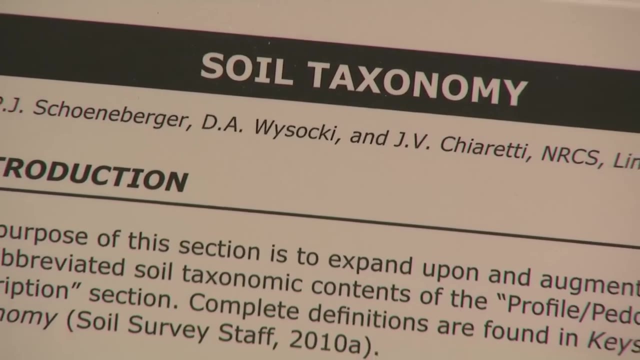 It is important to understand that genetic horizonation does not necessarily equate to diagnostic horizons. in soil taxonomy, Designations of genetic horizons express a qualitative judgment about the kinds of changes that are believed to have taken place in the soil. Diagnostic horizons are qualitatively defined features that are used to differentiate between 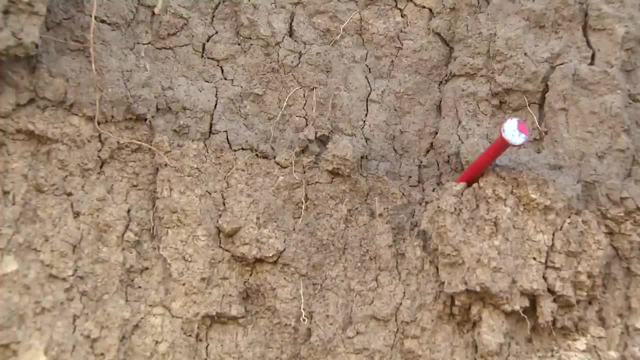 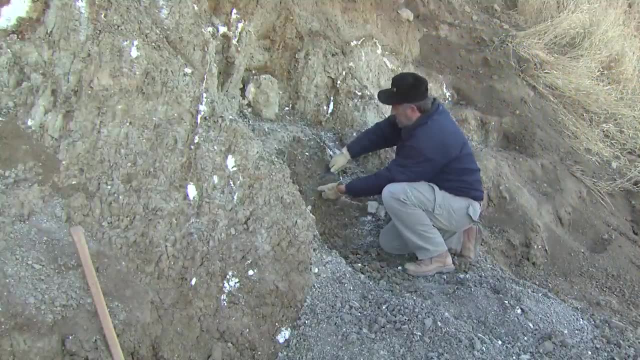 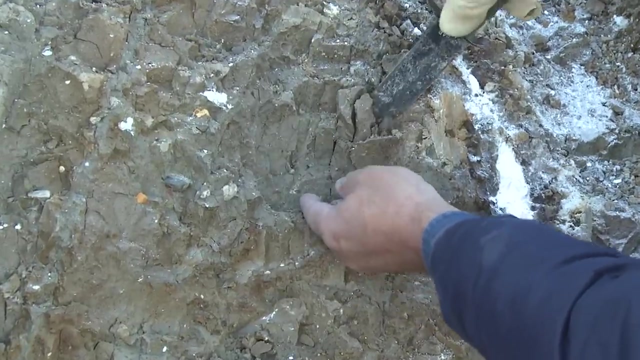 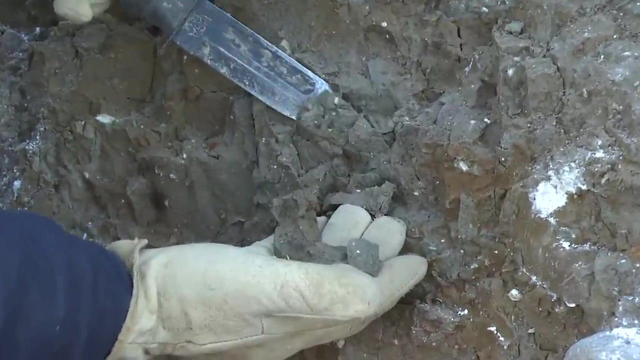 taxa. A diagnostic horizon may encompass several genetic horizons And the changes implied by genetic horizon designations may not be large enough to justify recognition of different diagnostic horizons. An experienced soil scientist can help you with the proper application of vertical subdivision of master horizons, recognition and description of discontinuities and the use of the prime. 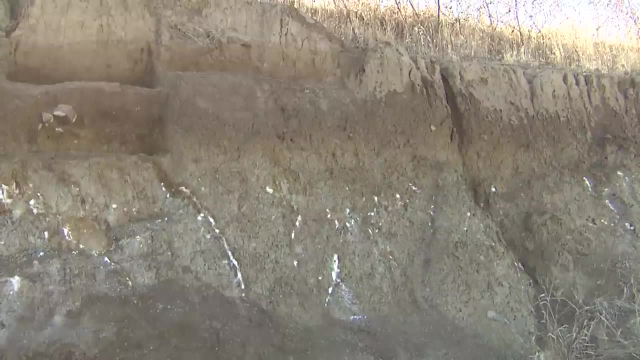 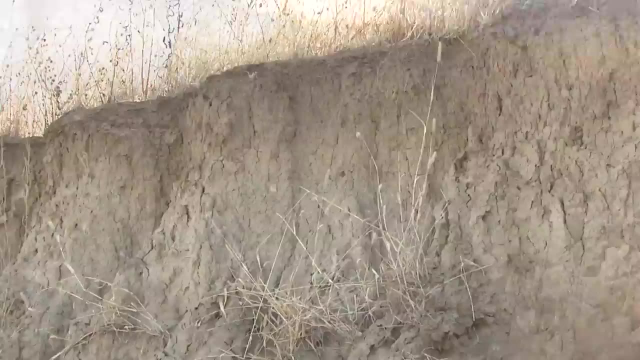 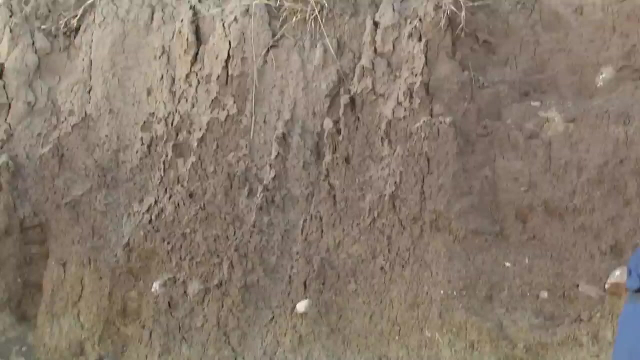 and caret symbols when applicable. The same can be said for recognizing and describing horizon boundaries in terms of distinctness and topography. Be sure to discuss alternative horizonations as possibilities and ask questions until you understand the horizon label descriptions. This job aid is designed to help you differentiate and identify soil horizons in the field, using 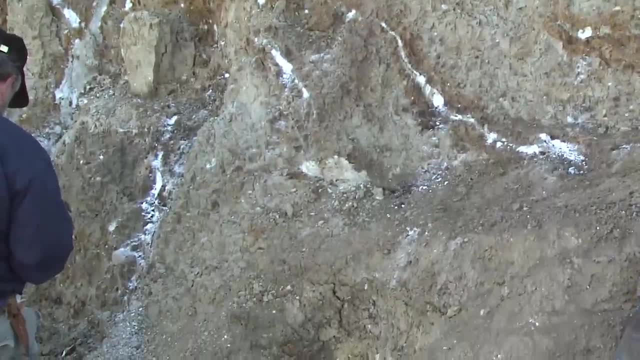 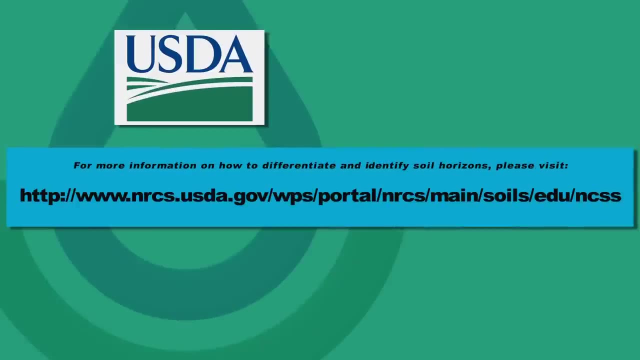 the National Cooperative Soil Survey standard methods. As with any new skill, proficiency comes with practice. For more information and tips on describing soils, please see our online NCSS training materials. For more information and tips on describing soil horizons, please visit our website NCSSgov. 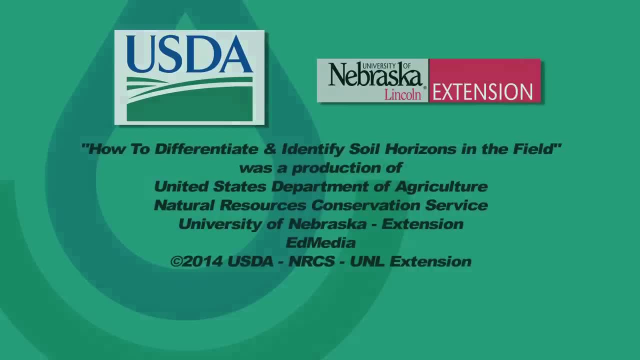 For more information and tips on describing soil horizons, please visit our online NCSS training materials. 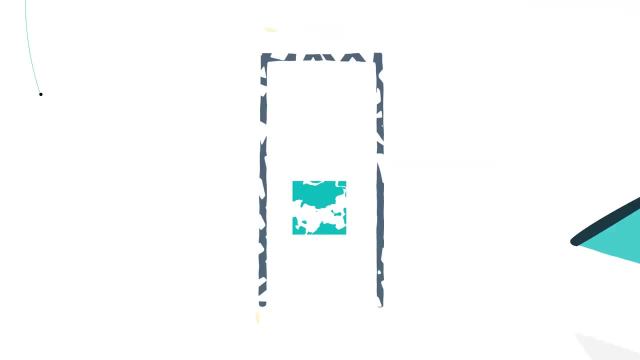 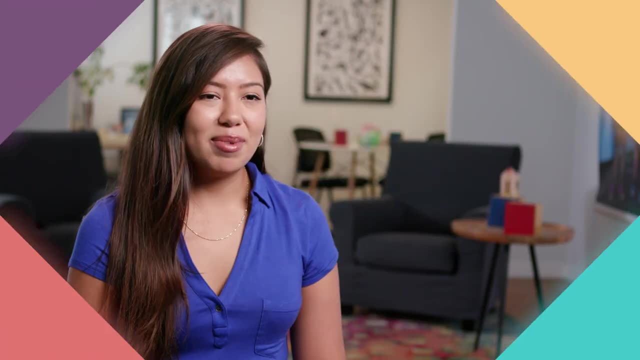 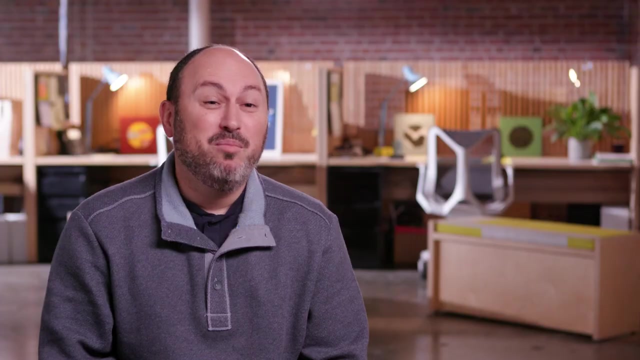 Hi everybody. my name is Gemma Bassoni and I'm the CEO of Discover Labs. I'm Jevon and I'm a CS student at UW Seattle. I'm Levar and I'm a software engineering manager at Airbnb. My name is Pan and. 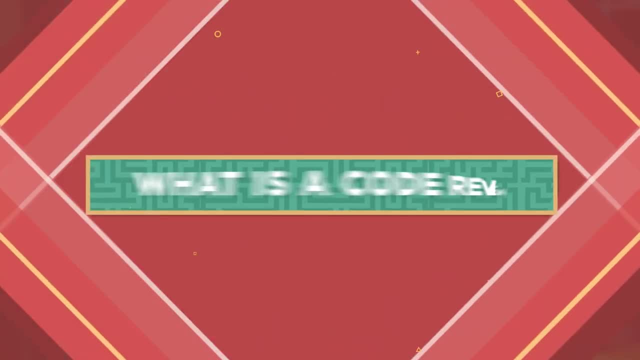 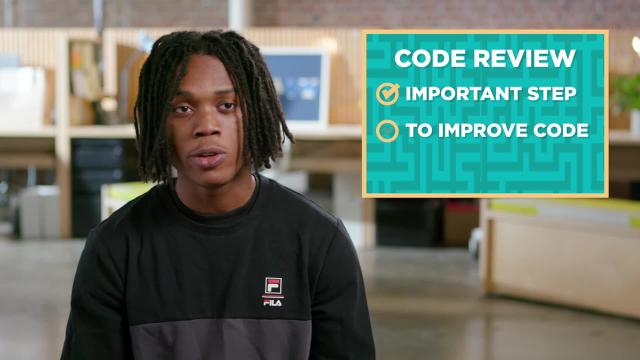 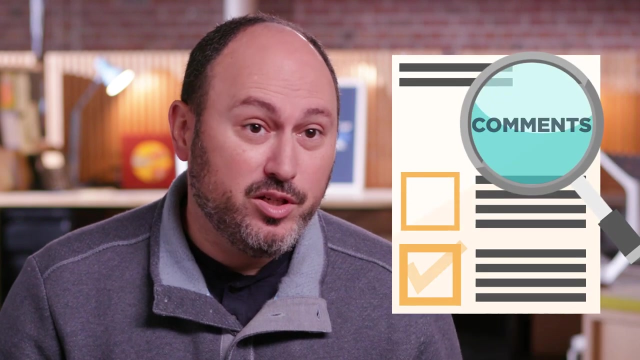 I am a software engineer at Xbox. It's probably one of the most important steps in pushing code: Looking for ways to improve it or ways to debug any problems that already might be there. You can go in and you leave comments and you have a conversation with the person who wrote the. 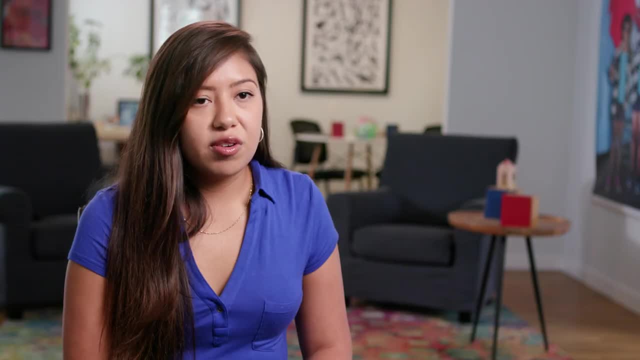 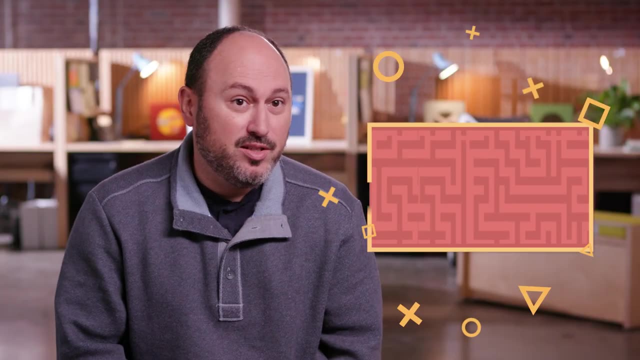 original code, And so it's having a second pair of eyes. Code reviews are important because they ensure the success of your code and your products. We don't always see our own errors. As the weeks and months roll in, I could see the evolution: I was writing better code and how the overall code 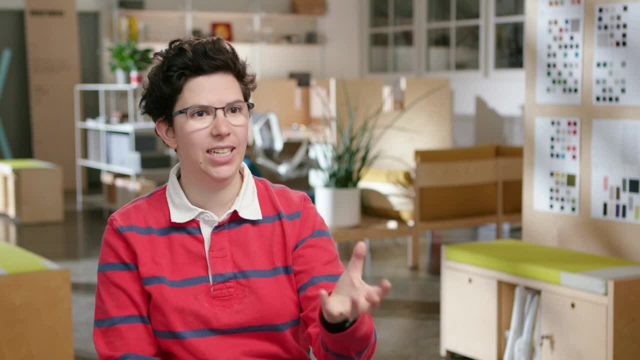 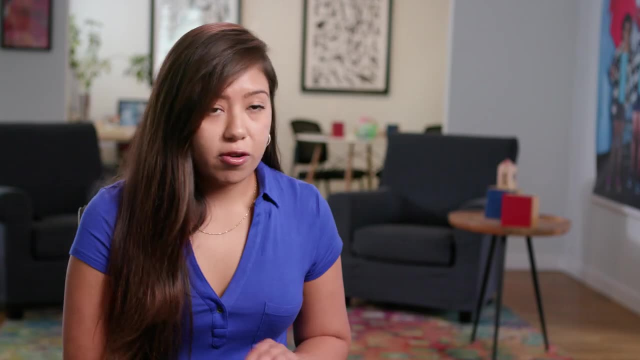 base was better. Every time I'm checking code on Git, I make a pull request and it mandatory must be approved by at least one person. It's a very powerful teaching tool. First run the code, make sure that everything actually works and then we'll sit down and look into it. I look. 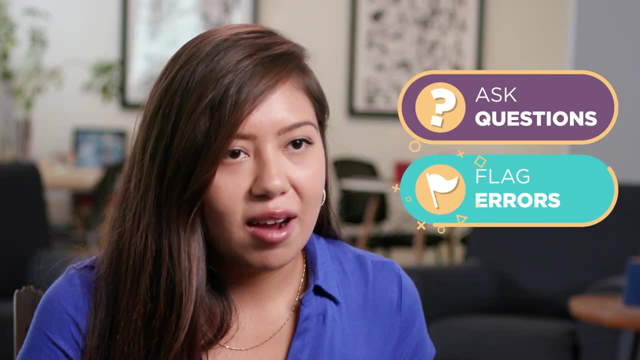 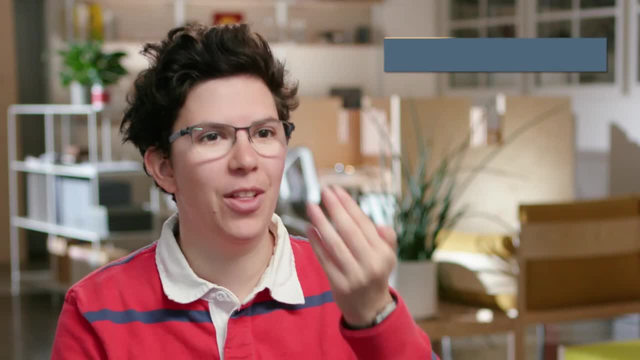 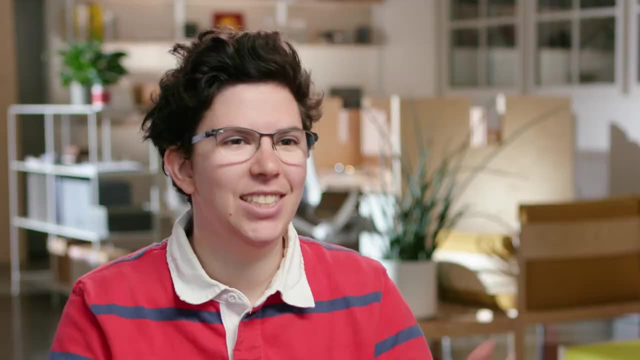 the code, and I look mainly towards logic, Learning a little bit more about the algorithm, the efficiency, the concept, the mental map, Any tests that could possibly break the program. It's a great way to learn- not the only way, but a great way. Code reviews.